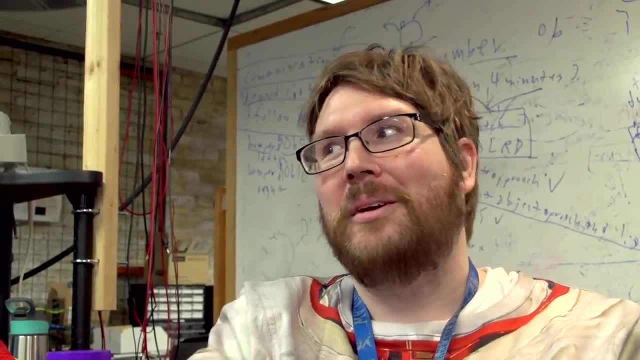 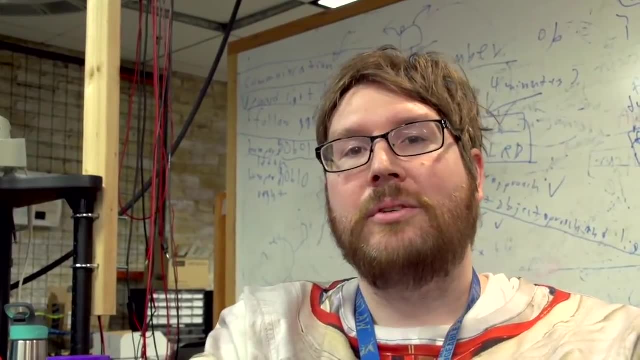 that have been developed since you know the somagraph that's been around forever. So we saw a thing called pulse transit time. Basically, what it is is you take your pulse at two different points in your body and then, through some physics, you can find your blood pressure. 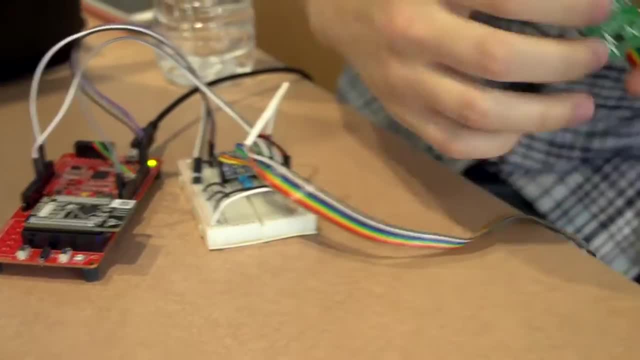 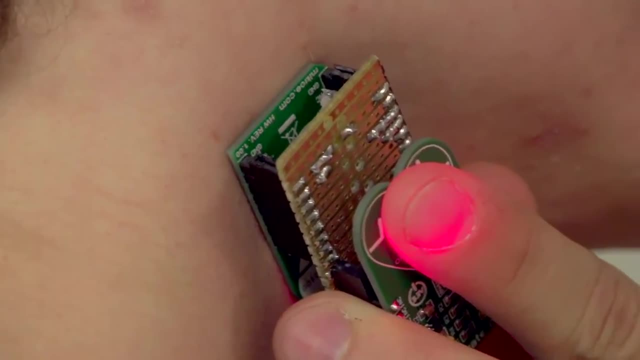 And then we decided: well, we could really make this compact into one single sensor, that you could just slip over your finger and then touch your neck at the same time, and we could get your blood pressure, and not only at just a single point. 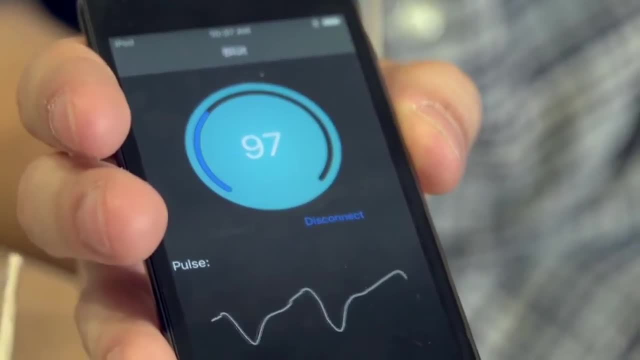 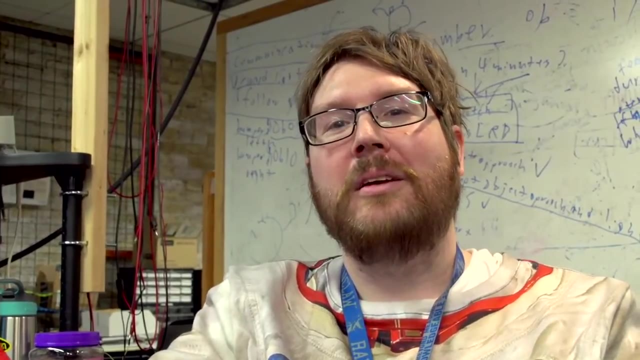 but a continuous blood pressure, which would be really useful for things like the sit-stand test, where you sit down and you stand up to see how your blood pressure changes. With this device, you simply just take your blood pressure every day, You do nothing else. You show up to your doctor- He already has it. 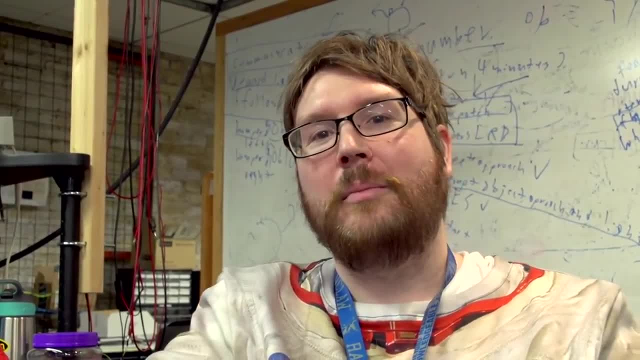 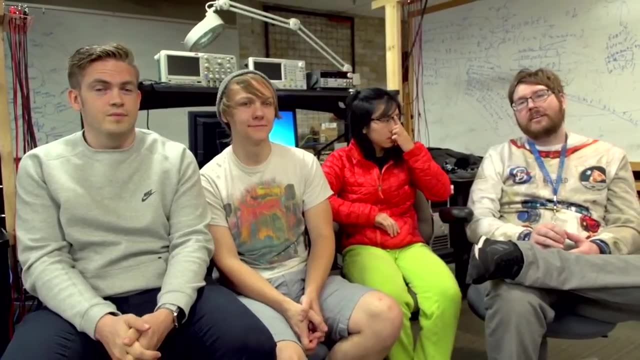 And you have a warning signal through the entire time if your blood pressure is raising over the days After graduation. we plan on continuing this project. We actually already started it in LLC and we want to take this product as far as we can, all the way to market, if possible. 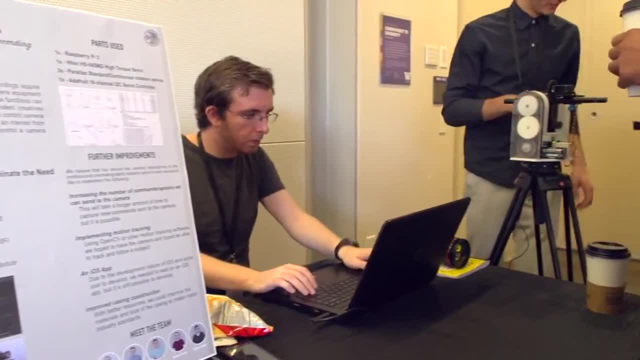 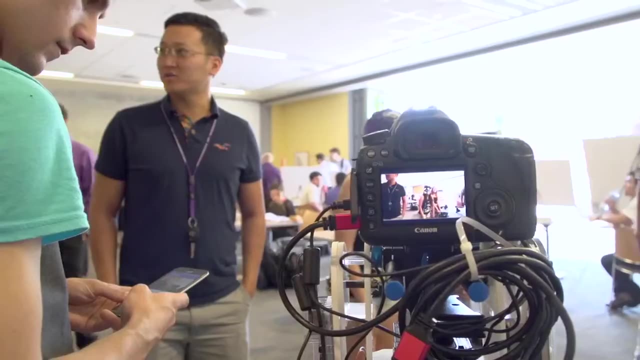 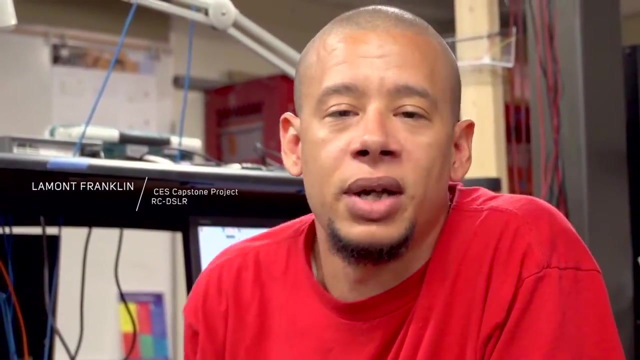 So our project is the DSLR remote. As you see, here we have the high-end DSLR camera. We're controlling the pan and tilt functionality, as well as the zoom and focus. We're doing that remotely. We intend on using an Android application connected to a Raspberry Pi remotely via Wi-Fi. 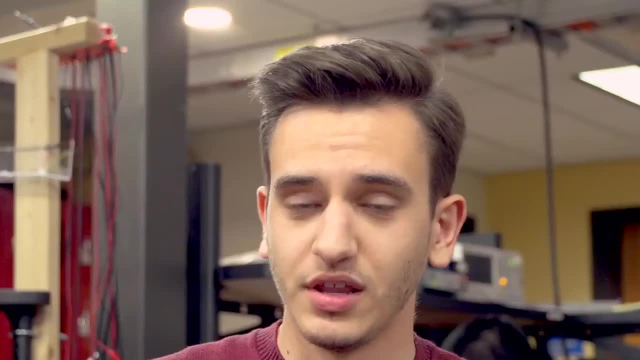 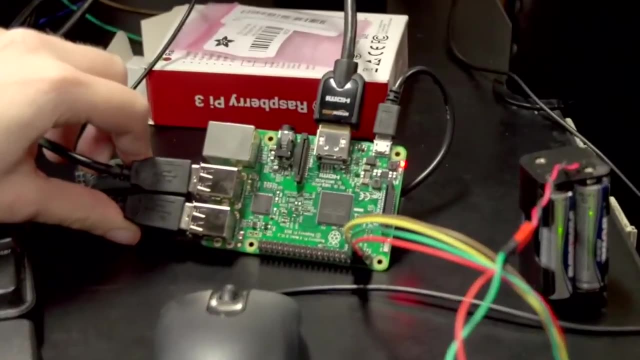 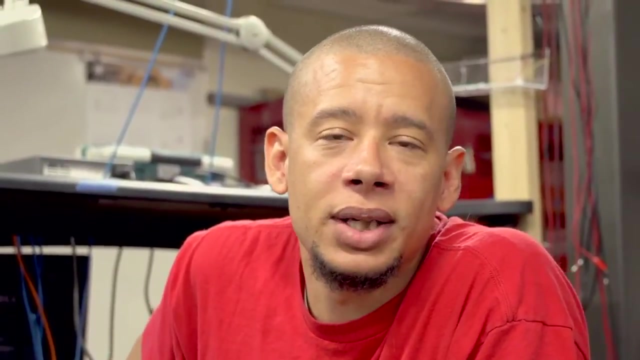 Our client is actually a House of Worship installation. The purpose for this device was actually to have the lead pastor be able to record himself while on stage, and this device allows for that. I'm finalizing this project after graduation, putting it into an actual consumer product. 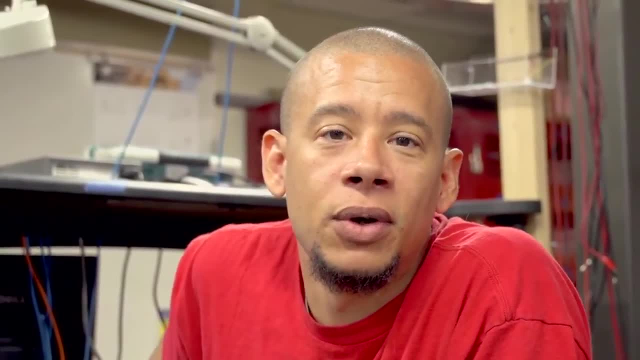 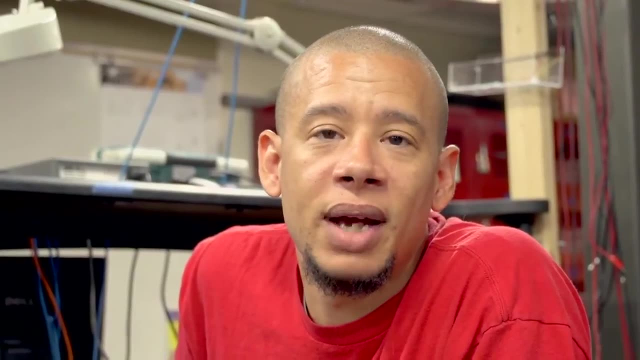 I have spoke with some of the staff over at Oracle who are also very interested in utilizing this product once it's completed. I think we'll probably start with a Kickstarter after we have our full proof of concept ready to go. I came to UW Tacoma because it was local. 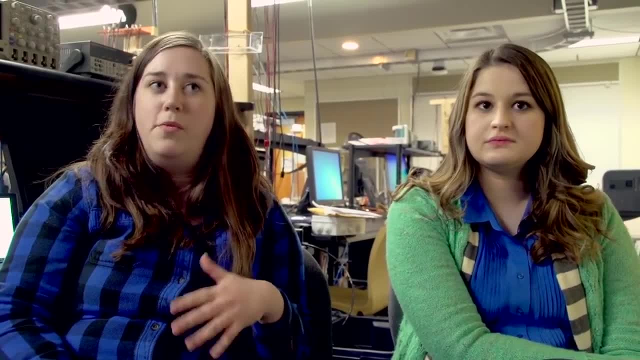 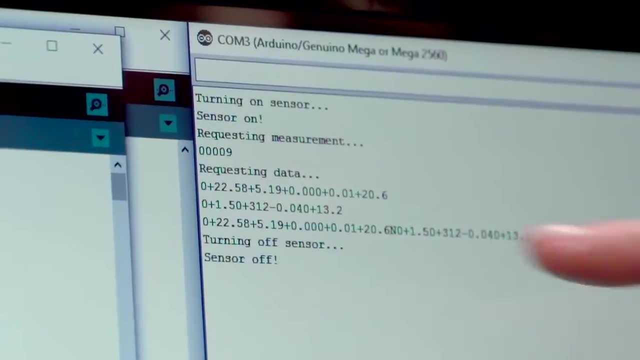 and I know they had the CES program here because I didn't want to just do software- And the program is very embedded systems focused and that's basically what we're building here. We're building an embedded system as software-led as possible, to control the hardware.